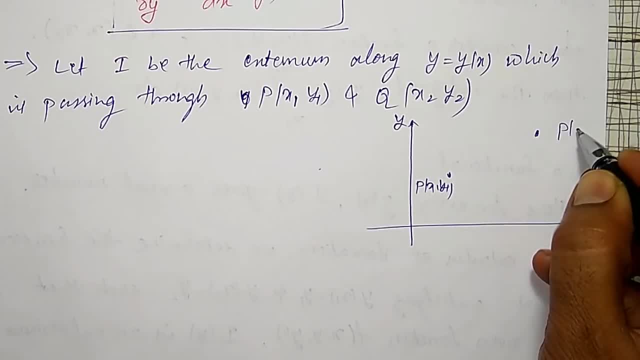 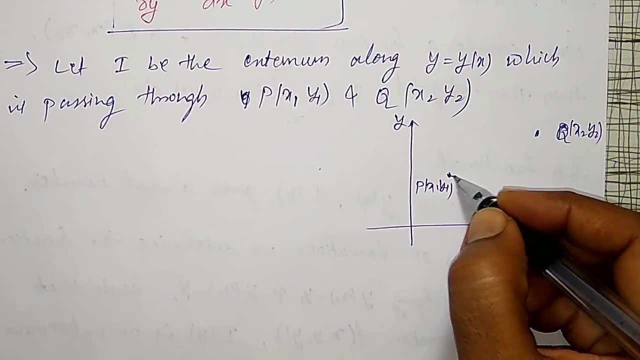 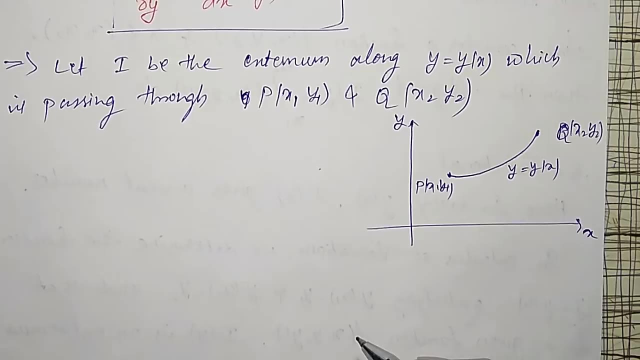 This is along y axis. This is along y axis: x1, y1. and another point: p, q, x2, y2,. okay, and I am considering a curve. okay, this is my curve: y equal to y of x. Now, to prove this, y is a extremum function. okay, well, extremum curve. 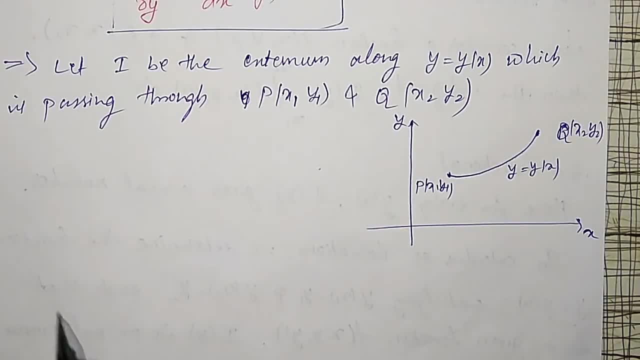 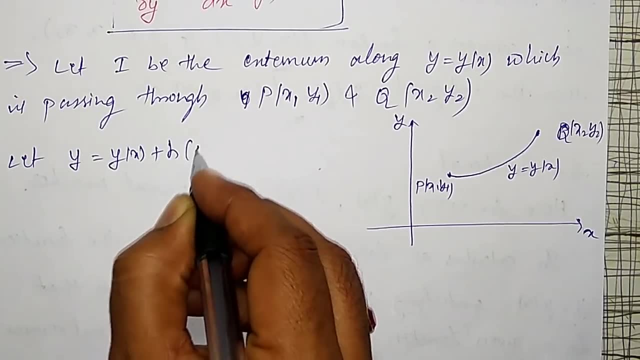 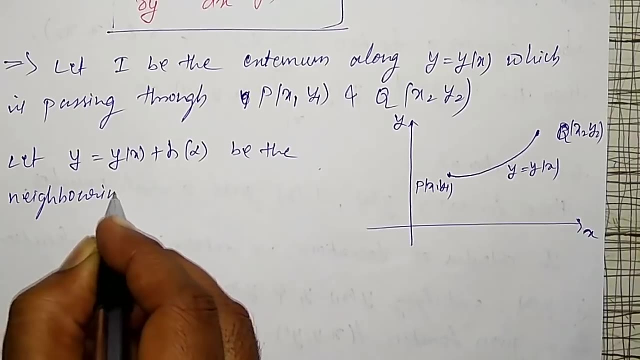 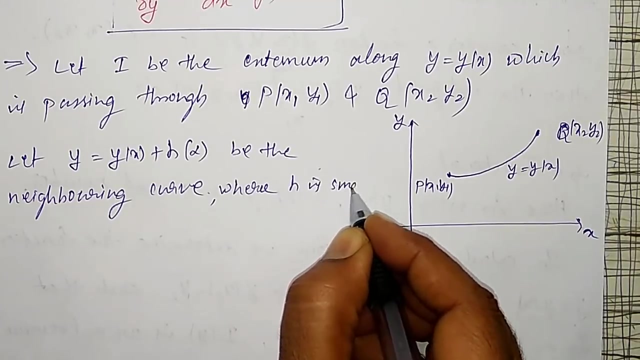 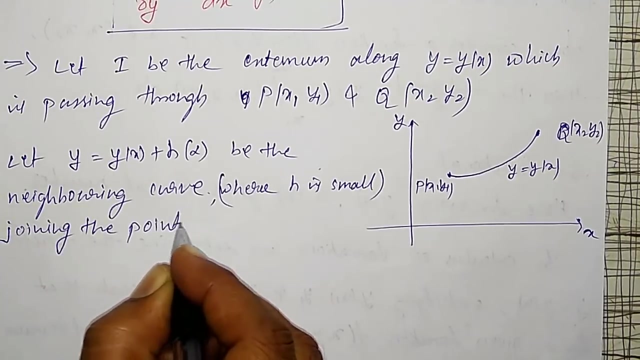 let me consider another neighboring curve. let y is equal to y of x plus h into alpha. be the neighboring curve. be the neighboring curve where h is a small quantity. okay, joining the point So that alpha of x. okay, so that I am considering the function: alpha of x1 equal to 0 and alpha. 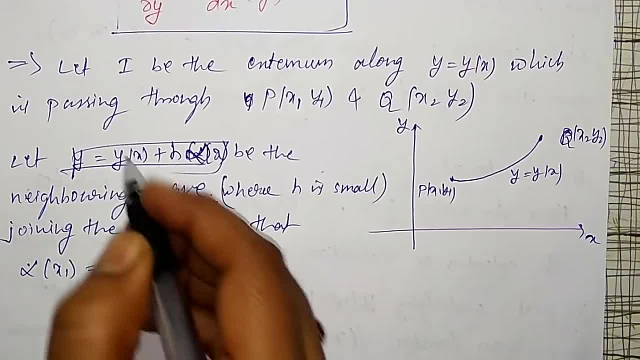 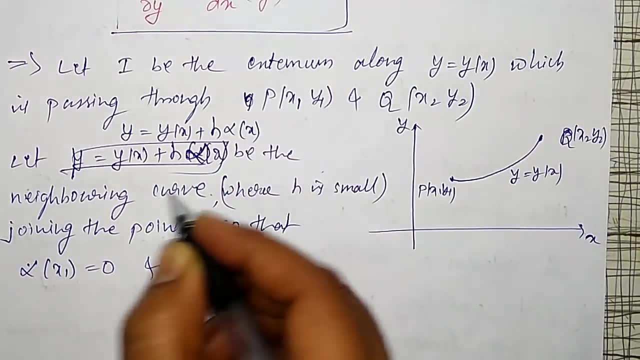 of x2 equal to 0, let me write this once again here. that is, y is equal to y of x plus h, of h into alpha of x. okay, another function I am considering Here in the diagram. let me show. 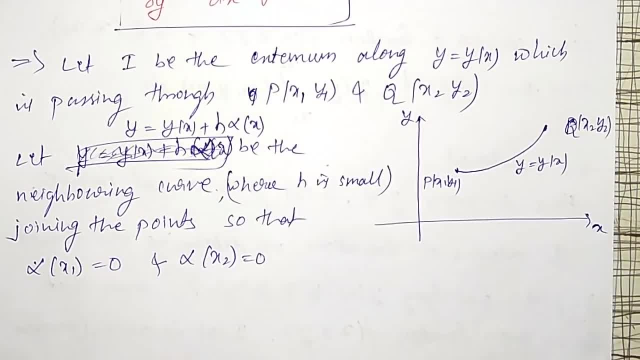 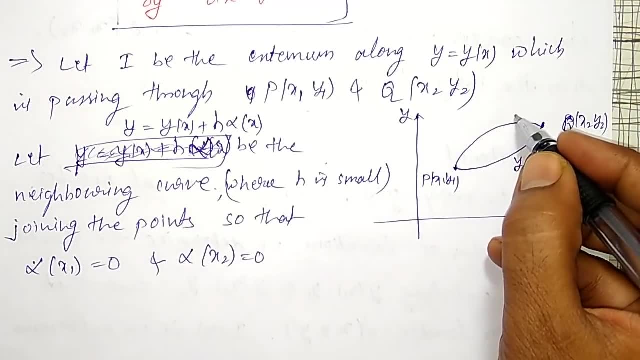 So that alpha of x is equal to y, of x plus h into alpha of x. okay, another function I am considering. I am considering another function. I am considering another function which is a neighbor to this curve and this is like this: this is my function: y is equal. 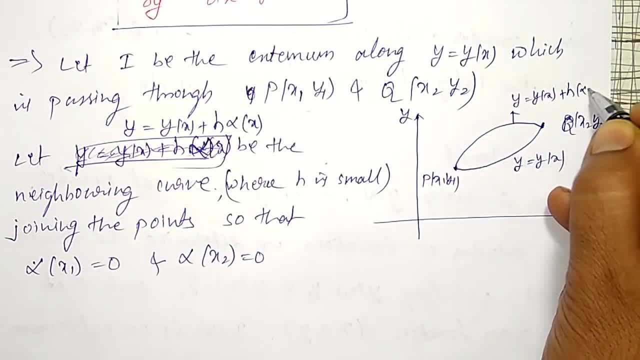 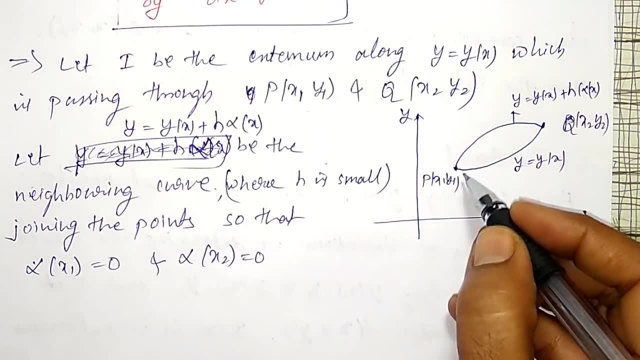 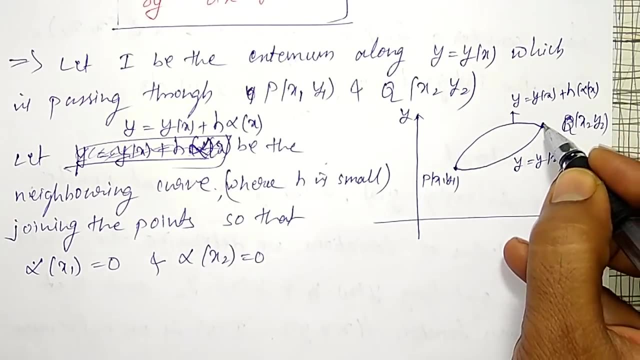 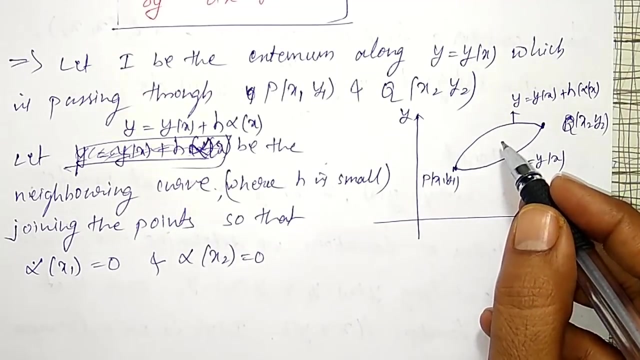 to y of x plus h into alpha x. okay, Now alpha of x1,. at this point, if you are substituting alpha of x1 in this, it will become y equal to y of x1.. same point. at these two points the curve is equal to same as y of x. okay, in other cases it is. 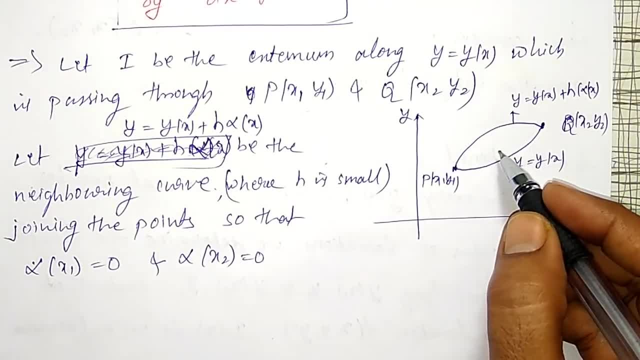 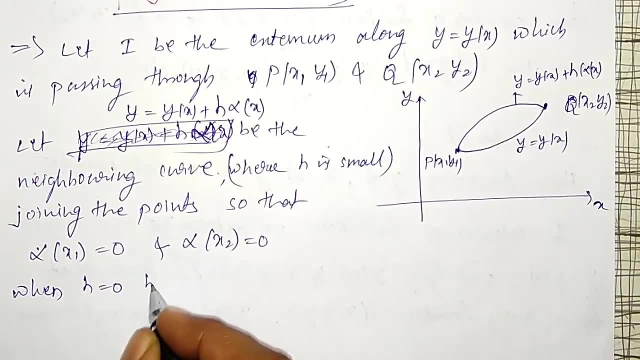 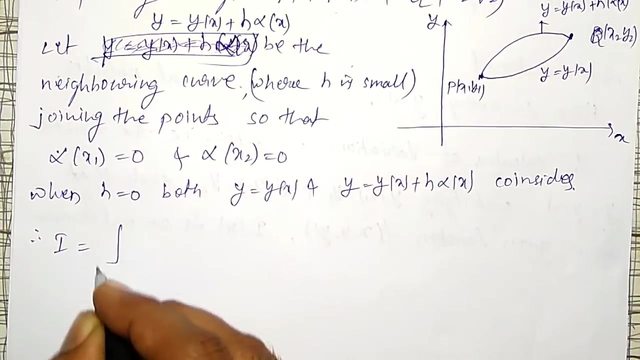 this one. okay, and this difference is the material h of h into alpha of x. okay, now h is equal to 0, both y equal to y of x and y is equal to y of x plus h into alpha of x coincides. okay, therefore, my integral, I equal to integration from x1 to x2, f of x, y, y will. 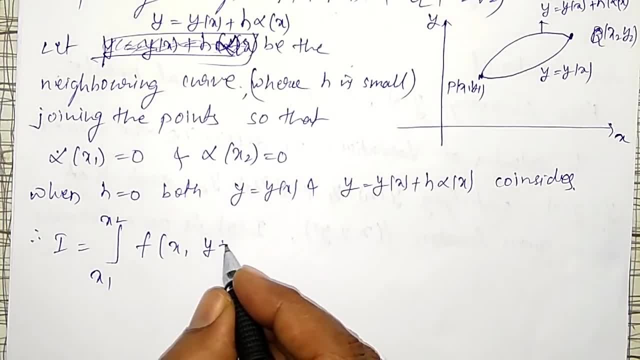 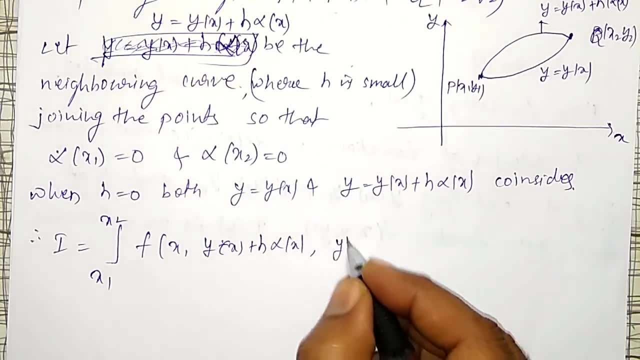 become now y of, except plus h into alpha of x comma. and what about y dash? y dash of x 2? You guessed it right, plus h into alpha dash of x. this is my dx. this is a function integral. i is an extremum at h is equal to 0. 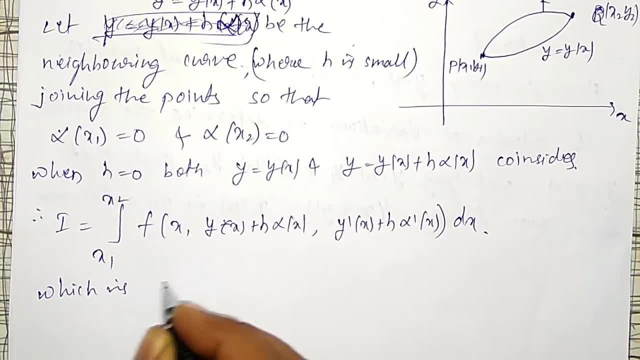 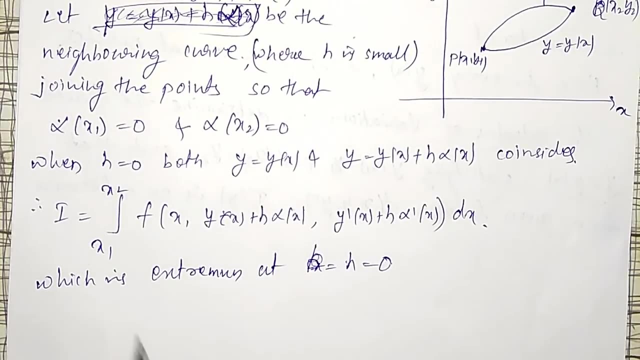 I have to prove which is extremum at h is equal to 0. this requires that after integrating this one, it is going to remain as a function of only h. here you are substituting for x equal to x1 and x2, and the function after integration is going to remain only a function of h. 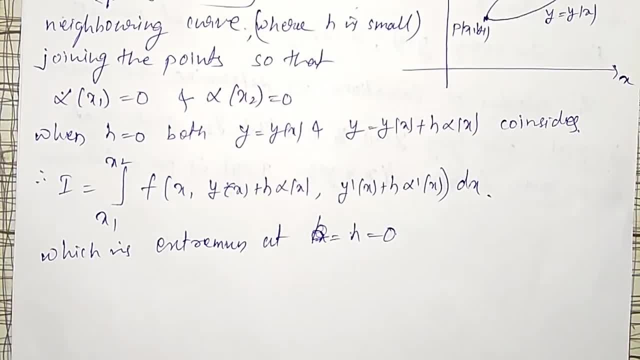 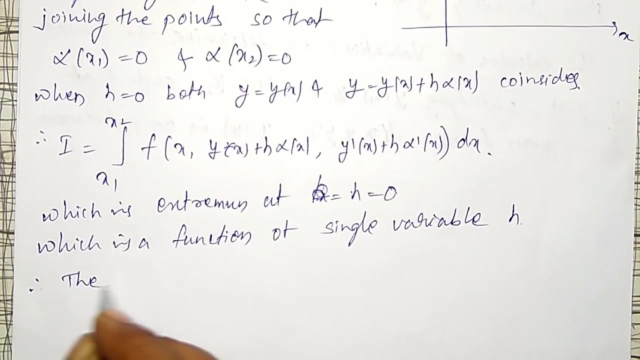 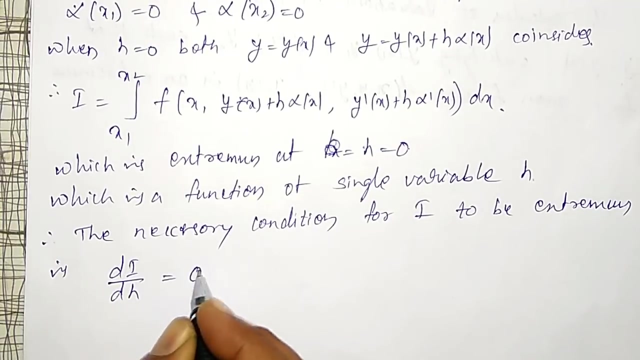 then the necessary condition, which is a function, function of function of single variable, single variable h, therefore the necessary condition, necessary condition for i to be extremum, extremum is d: i by d, h is equal to 0, treating i to be a function of h. here. 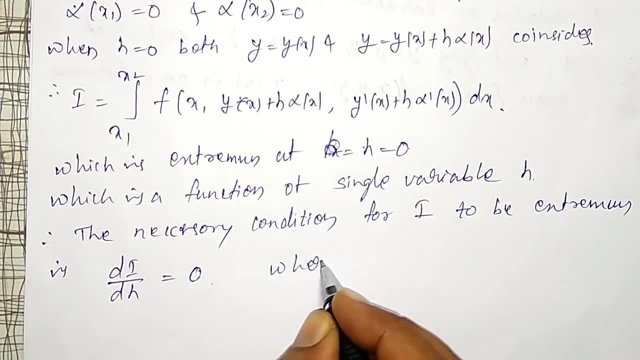 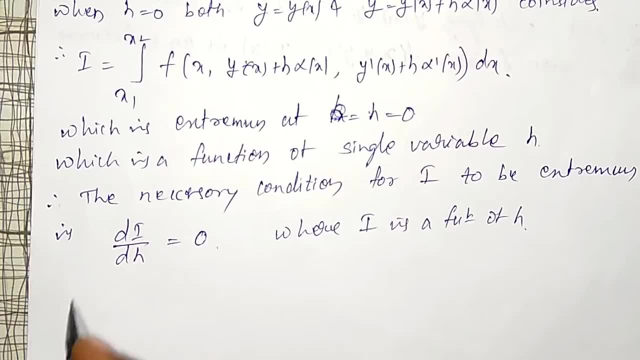 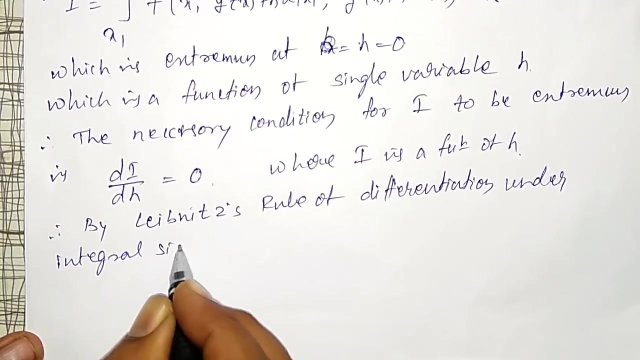 not treating it as a function of h, where i is a function of h. now, therefore, by by Leibniz rule of by Leibniz rule of differentiation under integral sign, differentiation under integral sign, the left hand side, i can write it as d i by d h equal to. 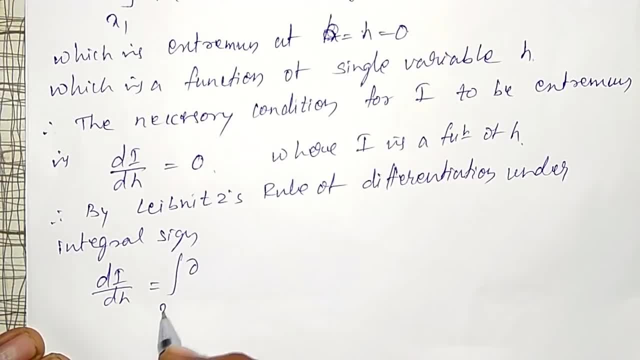 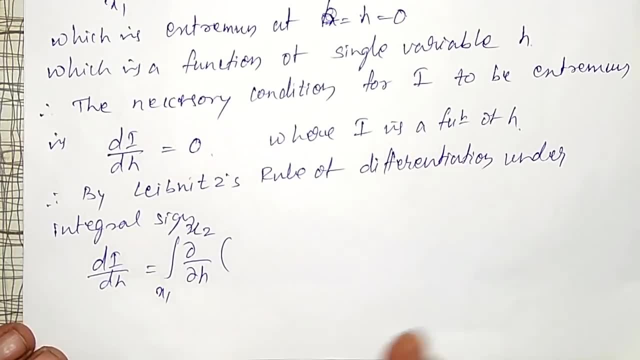 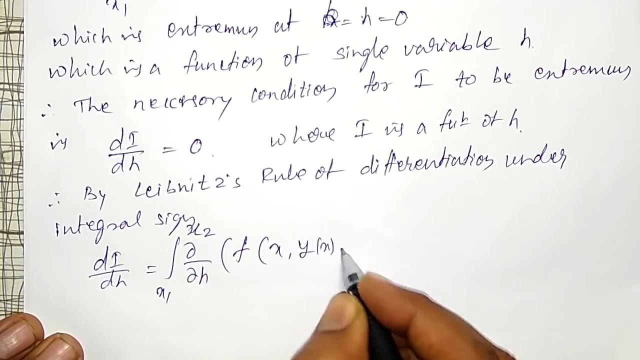 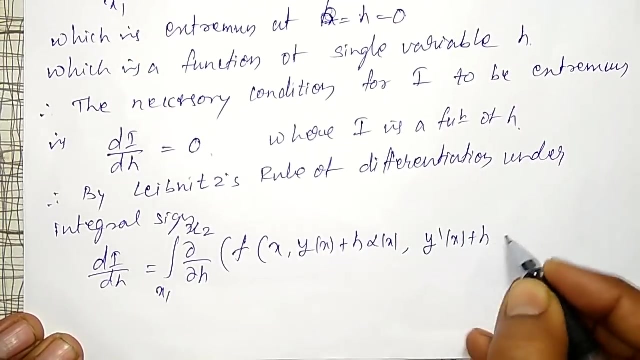 it is integration from x1 to x2 dou by dou h of partial derivative integration will become partial derivative of f of x comma y, of x plus h into alpha of x comma y, dash of x plus h into alpha, dash of x into dx. this one i have to differentiate partially. 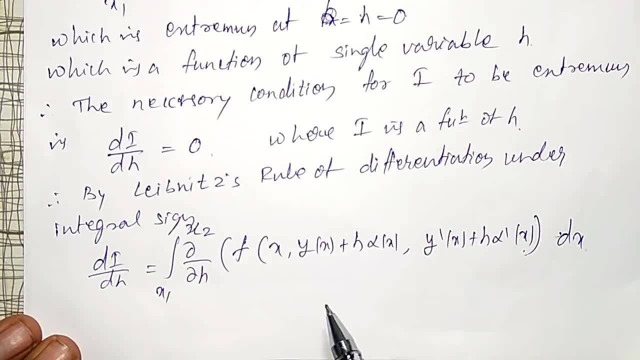 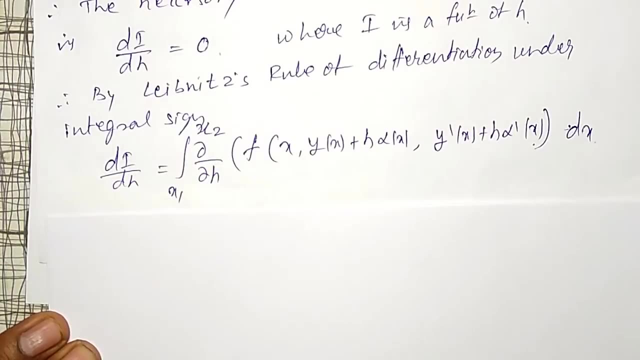 this one. i have to differentiate partially with respect to h here, while differentiating partially with respect to h. this is a function of x, y and y dash. ok, therefore i can write this one as d by d. h is equal to integration from x1 to x2. 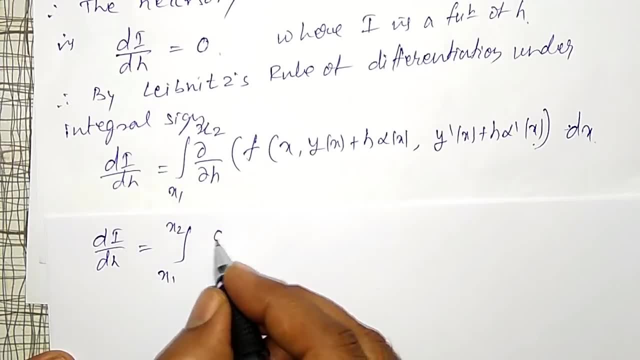 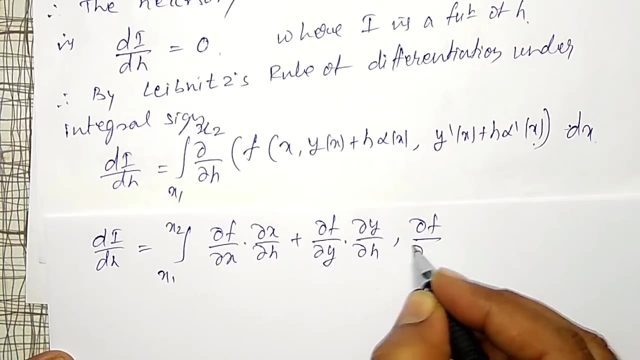 and partial derivative of this. i can write it as: dou f by dou x into dou x by dou h, plus dou f by dou y into dou y by dou h, comma. dou f by dou y dash into dou y dash by dou h, i can write equal to: 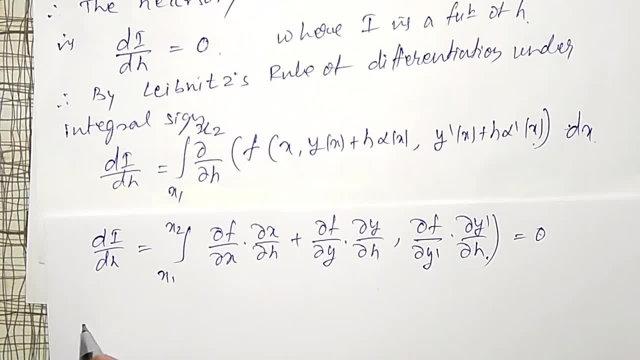 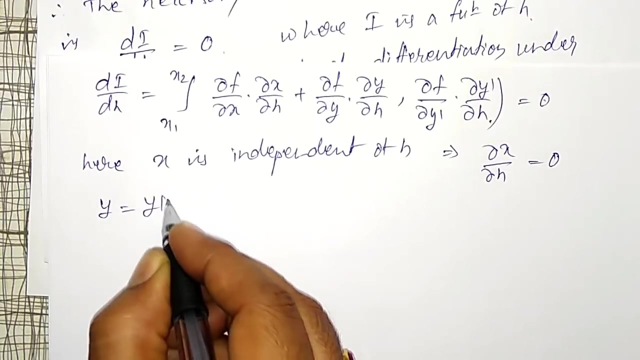 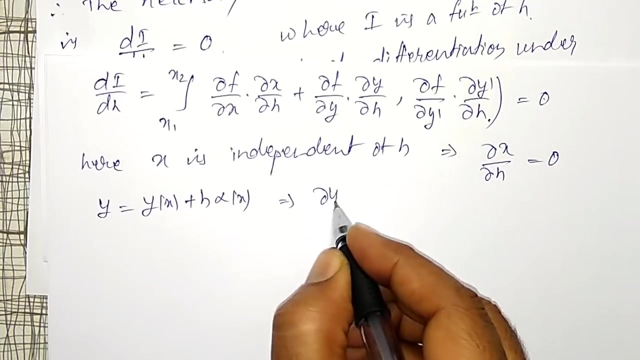 0. ok, and here x is independent of h. h is independent of h, which implies dou x by dou h is equal to 0 and dou y is equal to y of x plus h into alpha of x, which implies dou y by dou h is equal to. 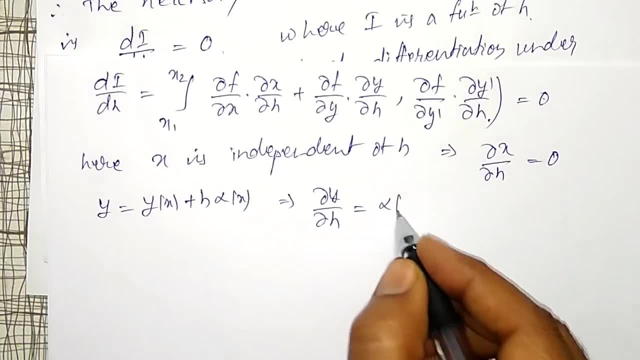 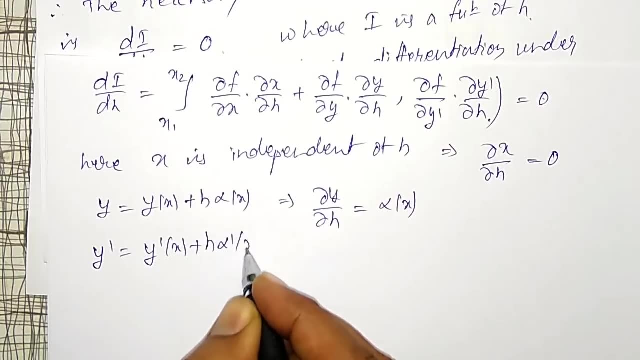 dou y by dou h is equal to alpha of x and y dash equal to y dash of x plus h into alpha dash of x, which implies dou y dash by dou h is equal to alpha dash of x. all these three i will substitute in this, therefore: 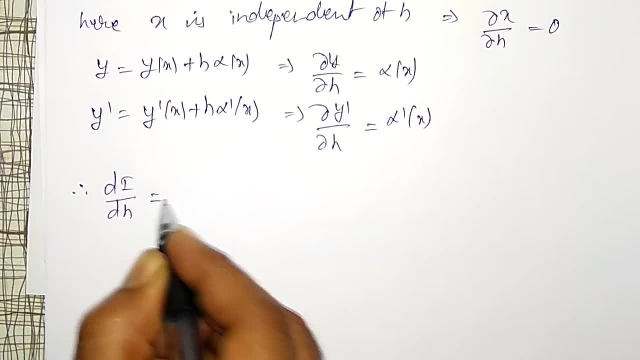 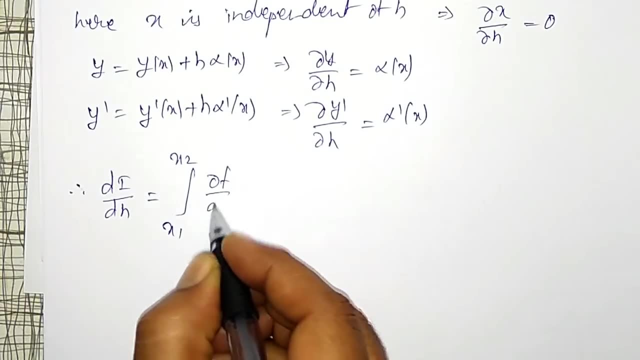 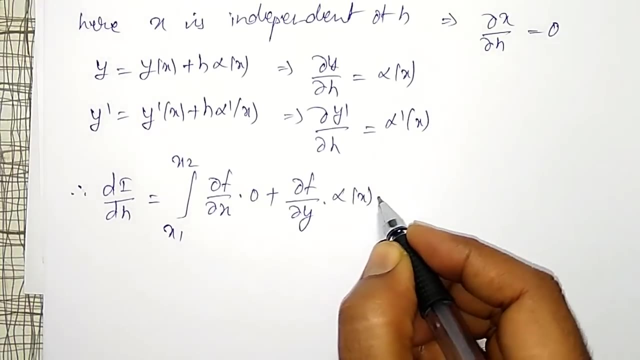 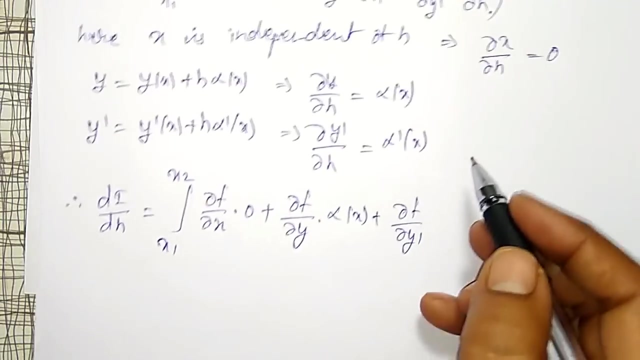 d i by d h is equal to integration from x1 to x2, first part. dou f by dou x into 0 plus dou f by dou y into alpha of x, plus dou f by dou y dash into dou y. dash by dou h is nothing but. 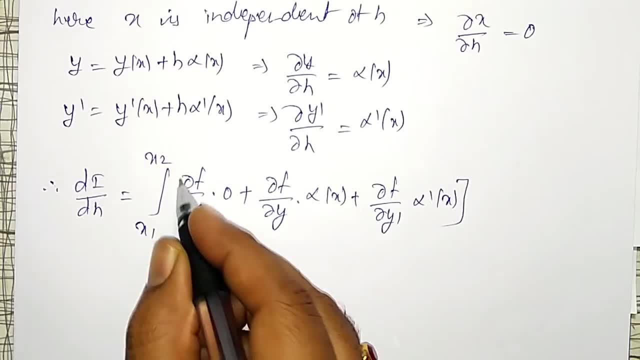 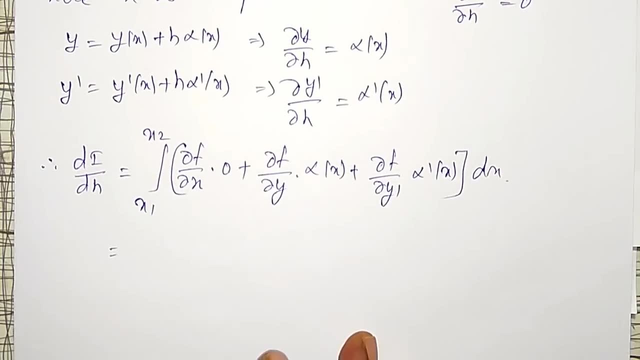 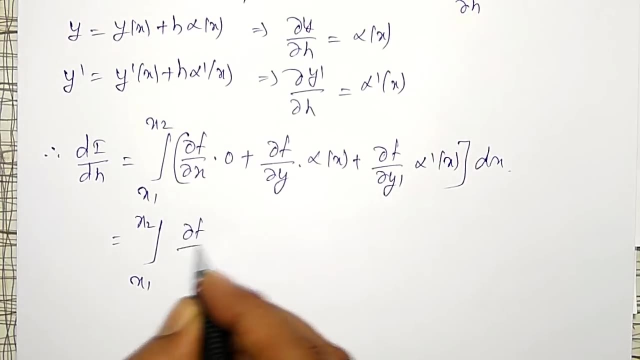 alpha dash of x into bracket dx. ok, now i have to integrate this one. ok, i will simplify this one and i can write this one as a integration from integration from x1 to x2, dou f by dou y into alpha of x plus dou f by: 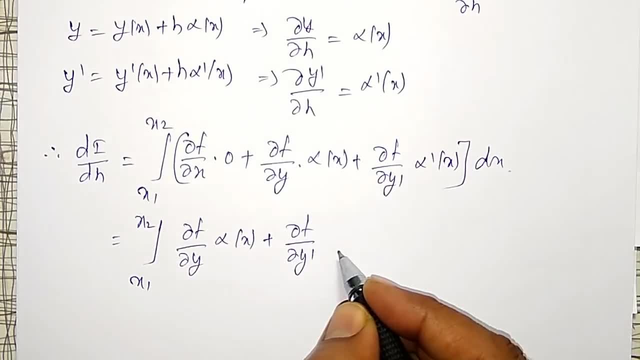 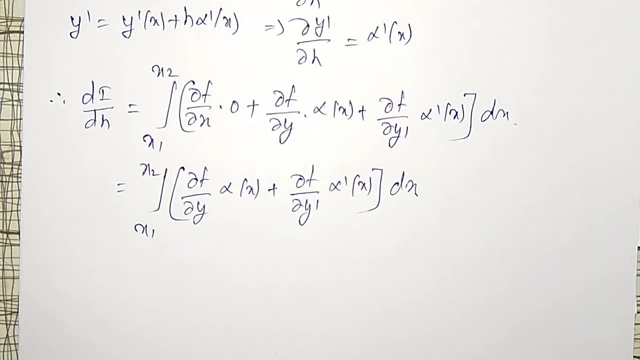 dou y dash into alpha, dash of x into dx. here, first term on the rhs, i will keep as it is. i will keep this one as it is and the second term only i have to integrate by parts. ok, integrating by parts. ok, integrating by parts. second term. 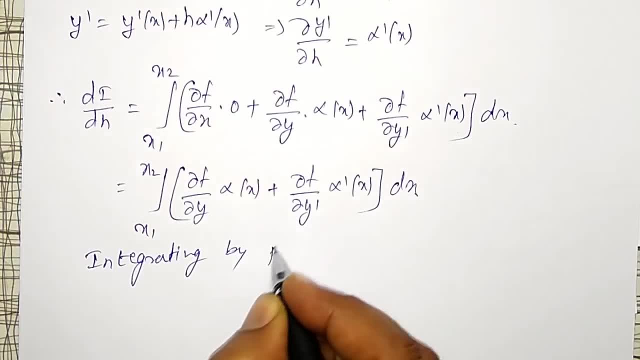 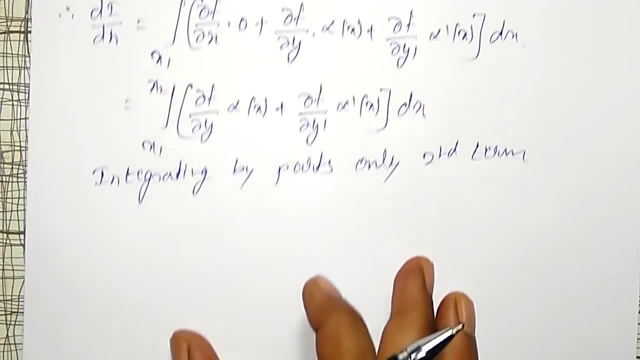 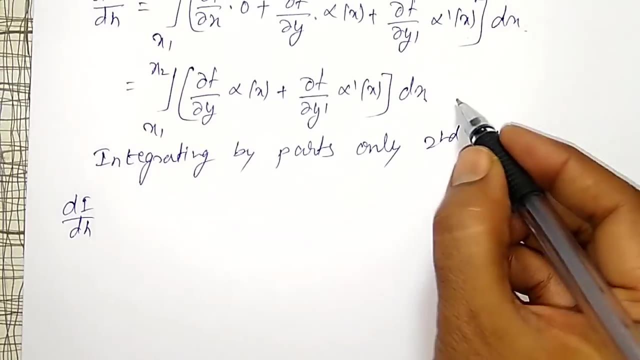 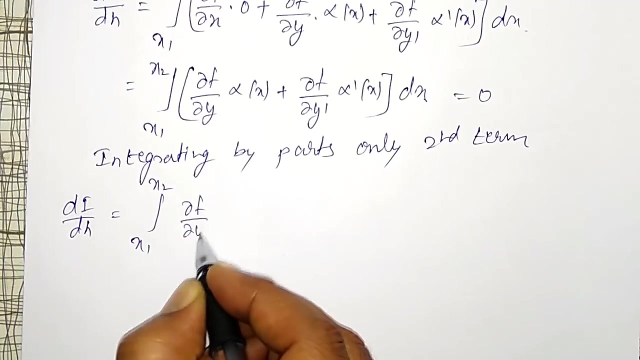 integrating by parts only second term. ok, then i am waiting. di by dh. ok, and that is equal to 0, it continues. it is equal to 0, equal to integration from x1 to x2, dou f by dou y, into alpha of x, dx, plus for this one. 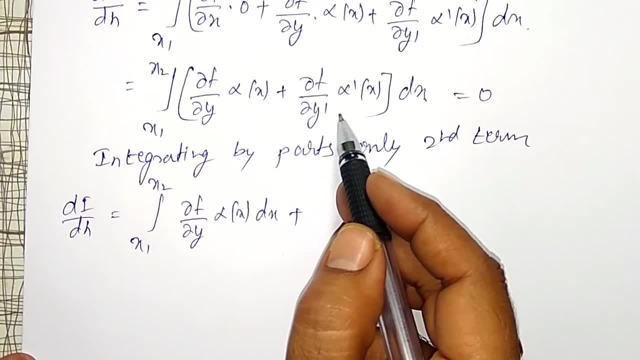 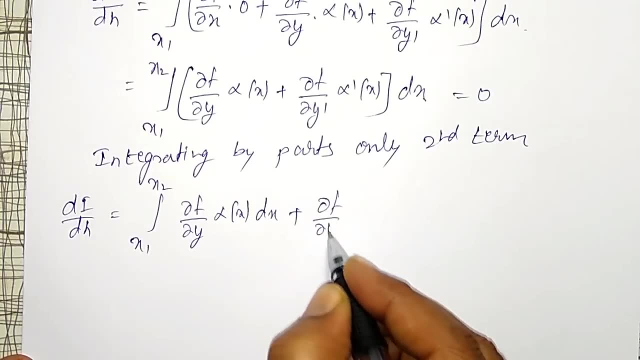 i have to integrate by parts. while integrating by parts, i will consider the first function, this one and this one. second function, that is, dou f by dou y, dash into integration of alpha, dash of x between x1 to x2 minus, minus integration of x1 to. 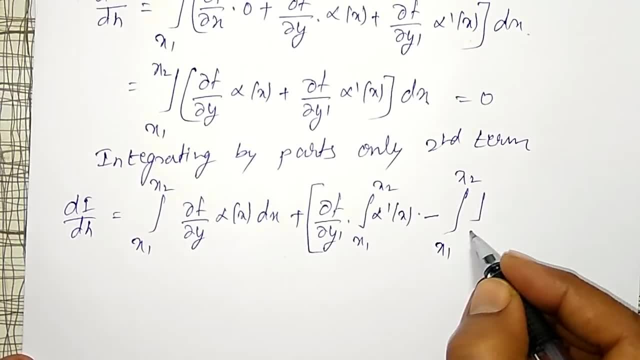 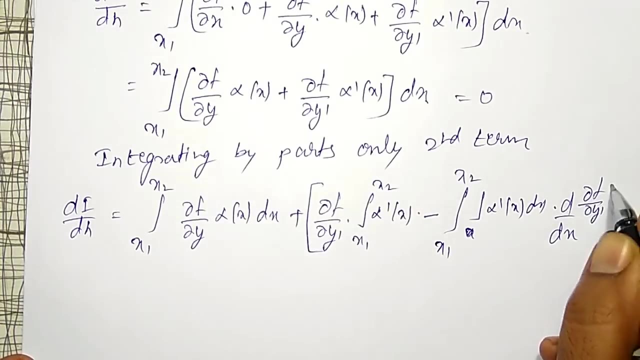 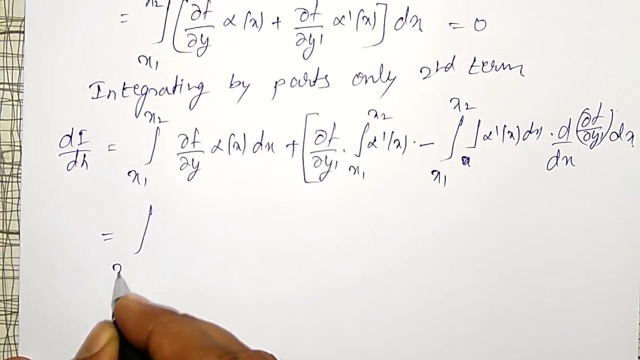 x2 into integration of this again, integration of ah, integration of alpha dash of x dx into differentiation of first function di dx of dou f by dou y dash into dx. simplifying this, what i am going to get here is integration from x1 to x2. 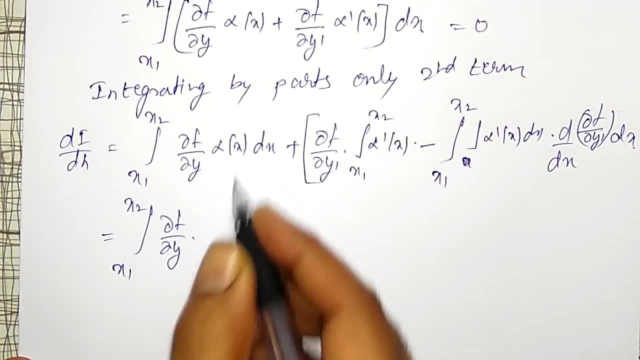 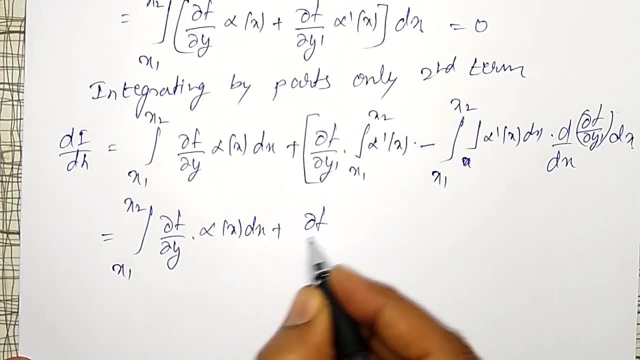 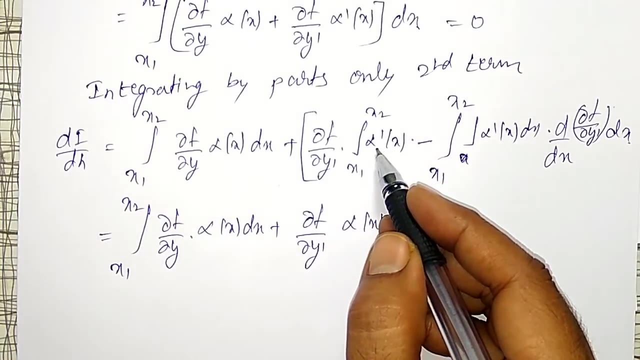 dou f by dou y into alpha of x dx plus, while integrating this, i am going to get dou f by dou y dash into alpha of x. differentiation of f dash is sorry. alpha dash is nothing but differentiation. its integration will become only alpha of x between the limits. 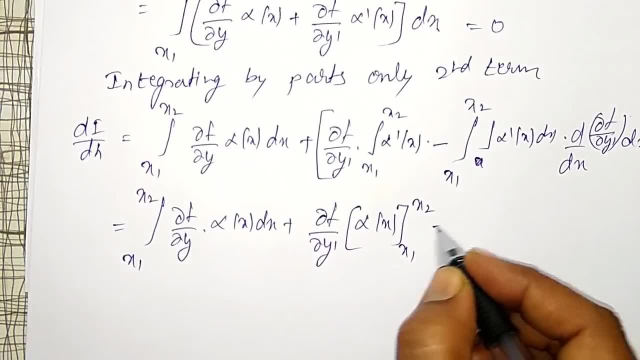 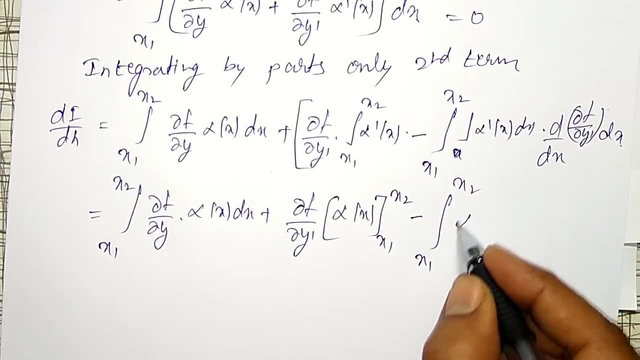 x1 to x2 minus. this one is nothing but again integration from x1 to x2. integration of alpha dash is nothing but again alpha of x into di, dx of dou f by dou y, dash into dx. that must be equal to zero again and here. 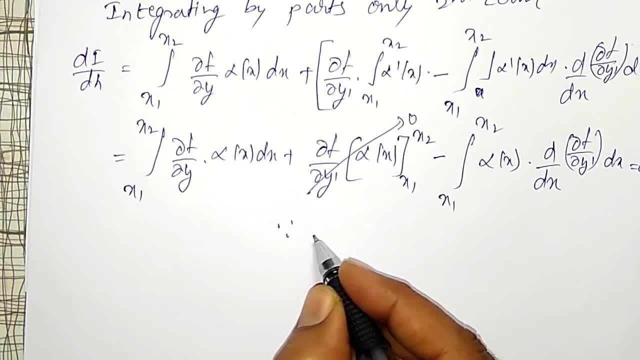 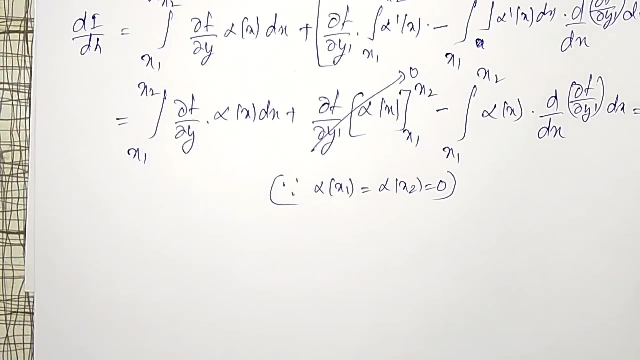 i can write this is equal to zero, since, okay, alpha of x1 if you substitute upper limit and lower limit and alpha of x2, equal to zero. for that reason, i can write this and remaining two terms together, i will write as: di y, dh, equal to. 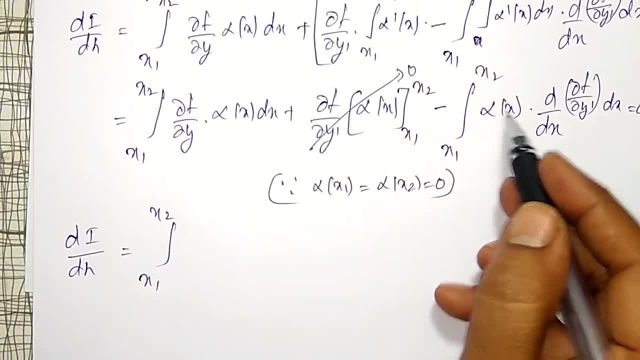 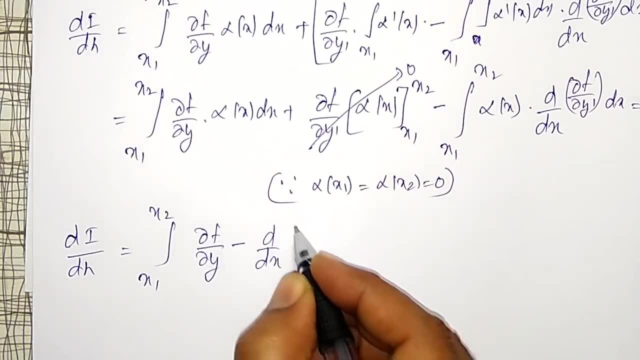 integration from x1 to x2. from these two terms, alpha of x, i will take common and i will write dou f by dou y minus dy, dx of dou f by dou y, dash into alpha of x, dx that must be equal to zero. and this integration. 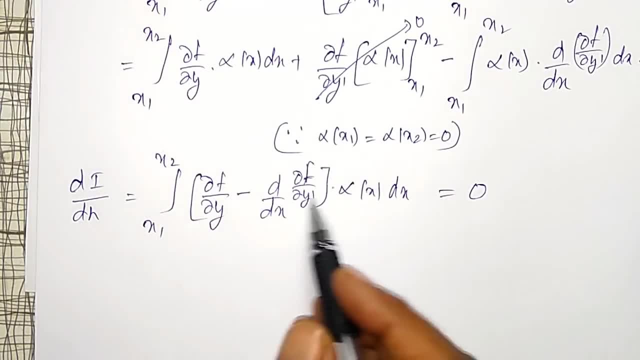 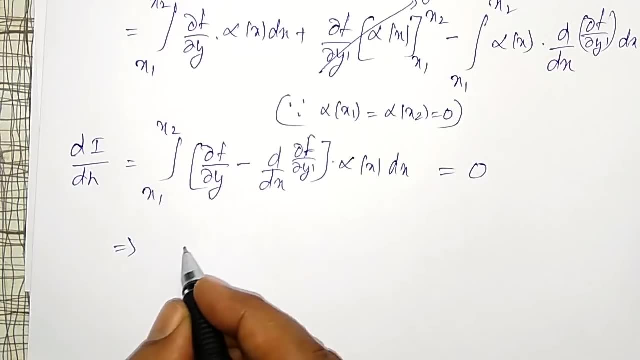 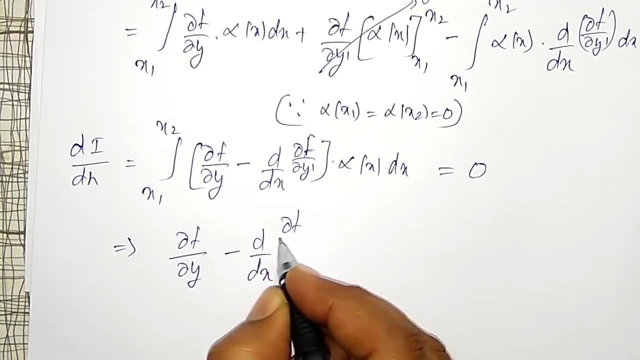 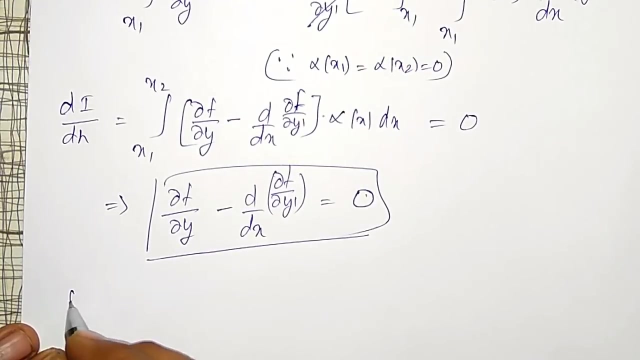 will become zero. alpha of x into dou f by dou y minus dy. dx of dou f by dou y dash must be equal to zero, which is the which is required. equation known as: dou f by dou y dash, which is the which is required. equation known as: